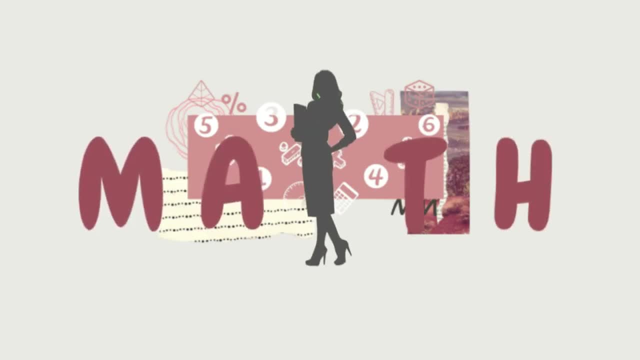 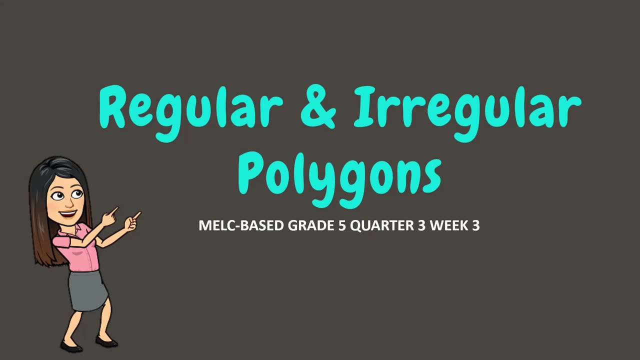 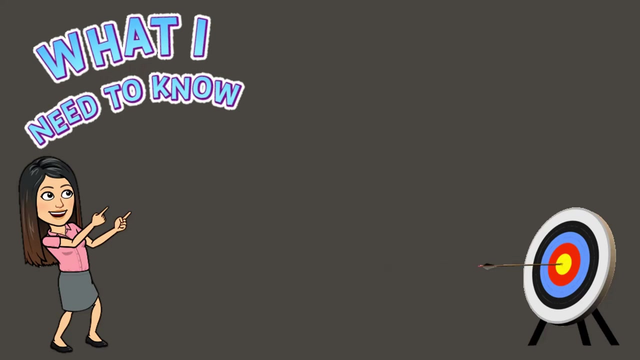 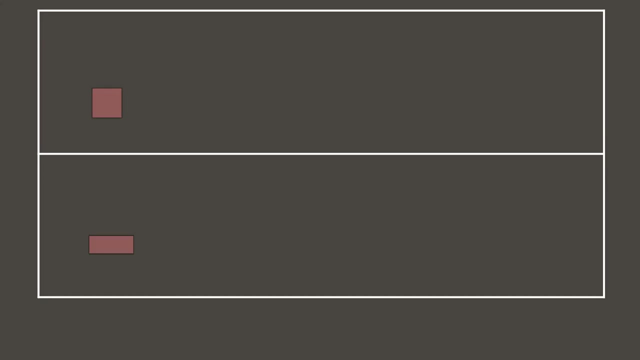 Regular and Irregular Polygons. Hello there, students. welcome back to my classroom For today's lesson. you will learn how to describe and compare properties of irregular and regular polygons. Let's go. Let's take a look at these figures. We have here two quadrilaterals: pentagons, hexagons, heptagons and octagons. 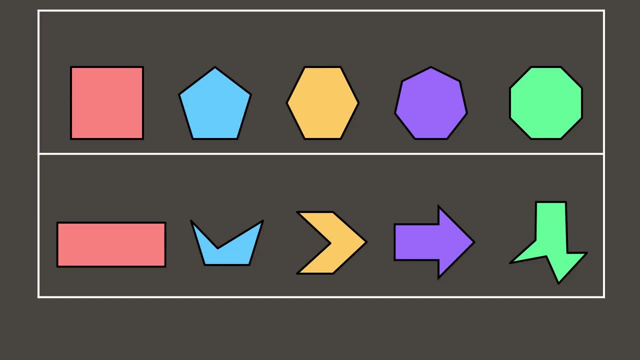 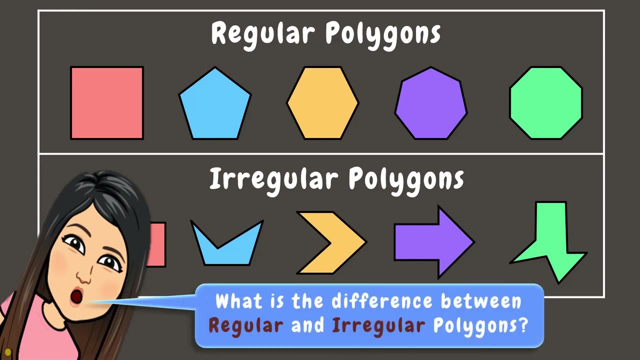 The first set of figures above are examples of regular polygons, while the second set of figures below are examples of irregular polygons. Now, by simply observing the two sets of polygons, can you tell the difference between regular and irregular polygons? Let's find out. 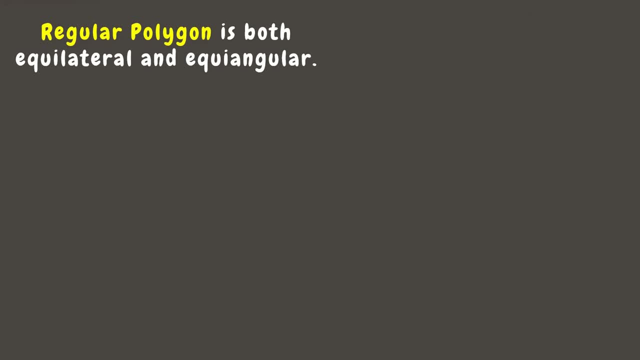 A regular polygon is both equilateral and equiangular. Equilateral means equal sides, while equiangular means equal angles. For example, a square has four equal sides. The tick marks on the line segments show that they are congruent or equal. 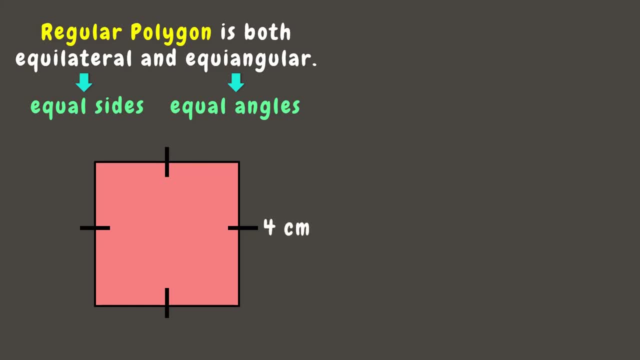 It means that when one side is 4 centimeters, the other side is also 4 centimeters long. This means the square is equilateral. Also, we know that the square has four right angles, which means it is also equiangular. 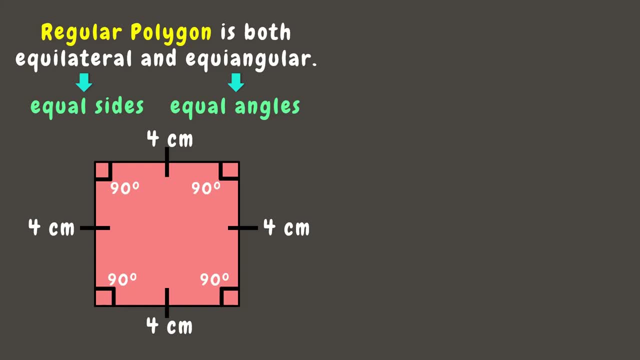 Since the square is both equilateral and equiangular, this means it is a regular polygon. Now, unlike regular polygon, a regular polygon has size and angles with different measure. For example, a rectangle-like square has four right angles. It means it is also equiangular. 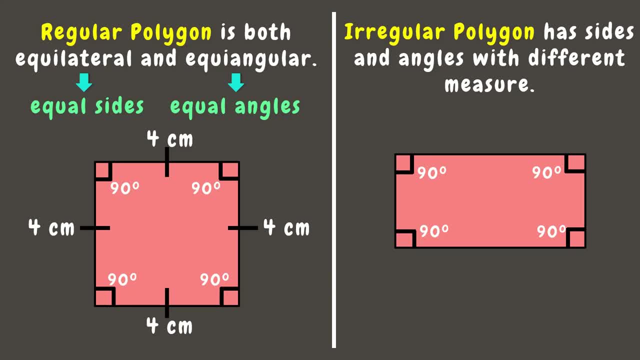 But a rectangle has only two pairs of sides equal. One pair is the length. It means that if one length is 5 centimeters, the other one will also be 5 centimeters long. Now the other pair is the width, which are also equal. 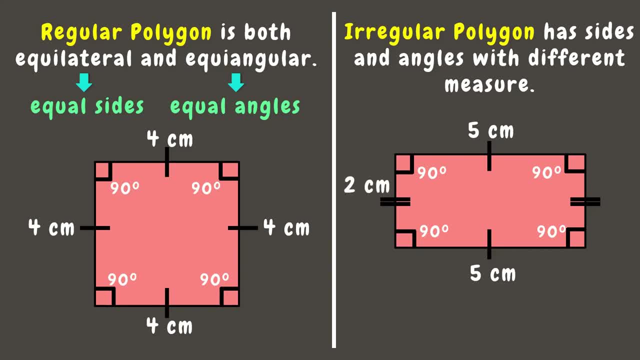 It means that if the width is 2 centimeters, the other one will also be 2 centimeters long. Now, the other pair is the width, which are also equal. Now, the other pair is the width, which are also equal. Now, even though a rectangle is equiangular, 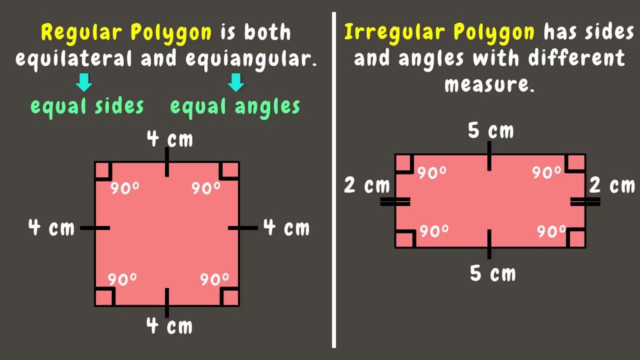 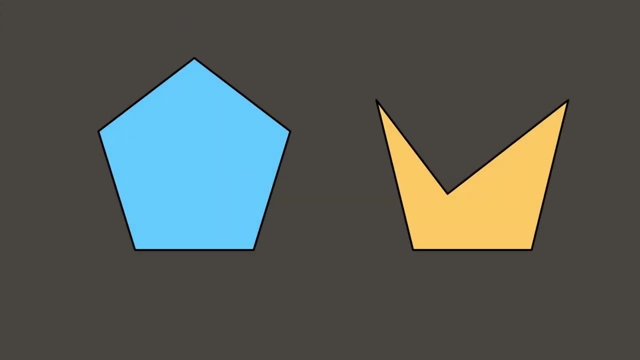 we can see that not all its sides are equal. This means rectangle is not equilateral. Therefore it is an irregular polygon. Let's have another example. By simply looking at these two polygons, we can say that the first one is a regular polygon. 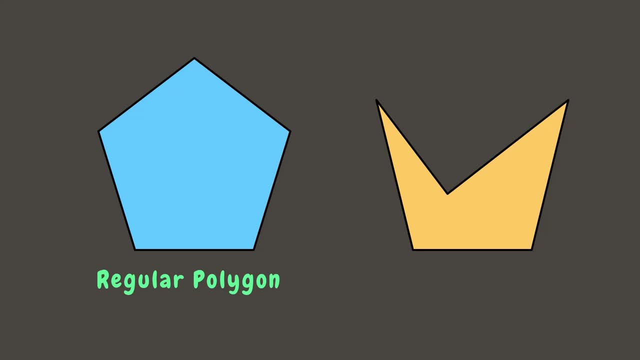 since it looks like it has equal sides. Since it looks like it has equal sides, we can say that the first one is a regular polygon, since it looks like it has equal sides and equal angles, While the other one is irregular polygon. 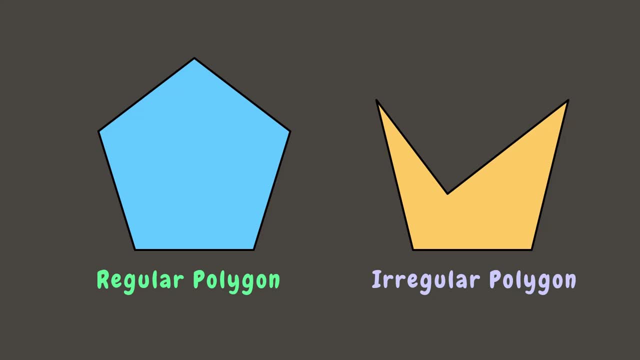 since it looks like its sides and angles are not equal. Since this polygon has 5 sides, we can call this as a regular pentagon, While the other one would be irregular pentagon. Let's go to the next one. Which one do you think is a regular or irregular polygon? 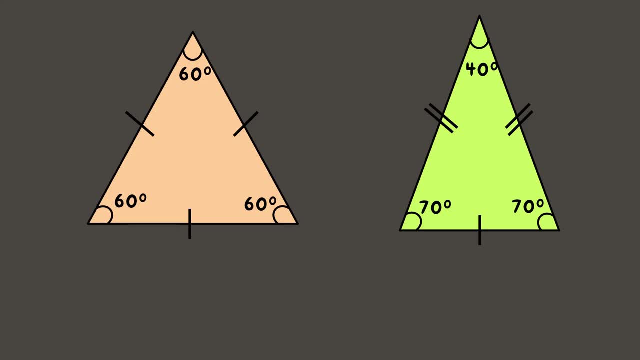 Which one do you think is a regular or irregular polygon? Which one do you think is a regular or irregular polygon? In the first polygon, we can see that the tick marks on the line segments are the same, which means they are equal. Therefore, it is equilateral. 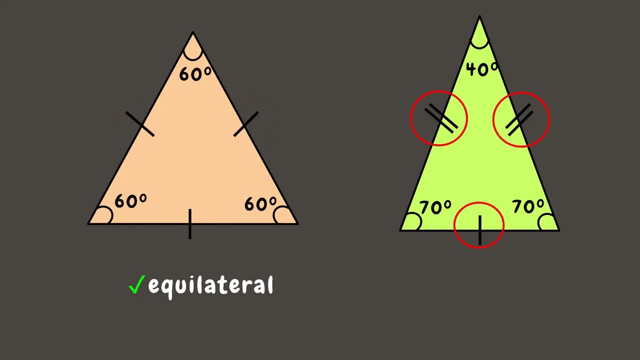 While on the other one we can see that only two sides have the same tick marks, which means only two sides and not all are equal. Therefore it is not equilateral. On the first triangle, all angles measure 60 degrees, Therefore it is equiangular. 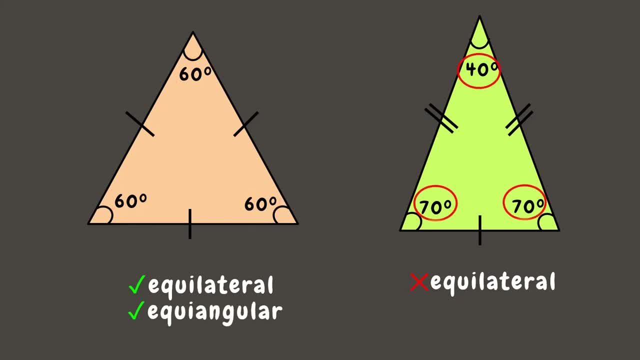 While the other one has only two equal angles, which is 70 degrees. Therefore, it is not equiangular, Since the first triangle is both equilateral and equiangular, this means it is irregular polygon, While the other one is irregular polygon. 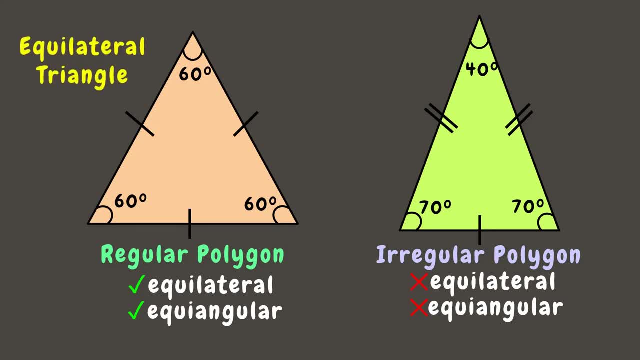 A triangle with all sides are equal is called equilateral triangle. Remember that all equilateral triangle is also equiangular triangle- While the other triangle, where only two sides are equal, is called isosceles triangle. Let's go to the next one. 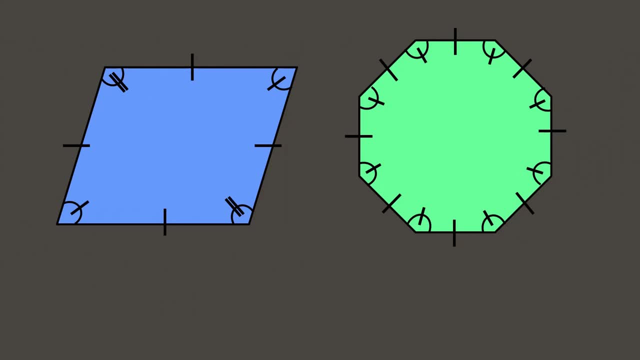 Again, let's find out which one is a regular and irregular polygon. The first polygon has four equal sides, Therefore it is equilateral. Also, the second one has eight equal sides, which means it's equilateral. Now we can see that the first polygon has two pairs of congruent angles. 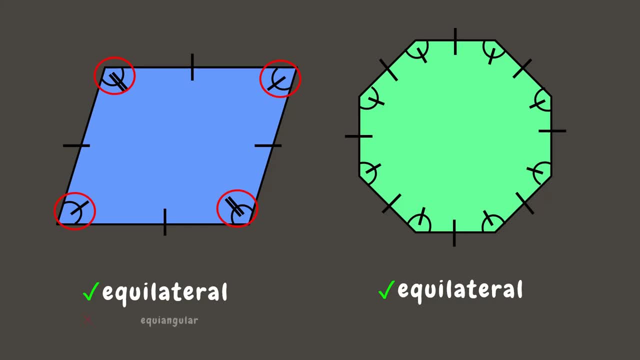 But not all are equal. Therefore it is not equiangular, While the second one has eight congruent angles, Therefore it is equiangular. Now, since the first polygon is not both equilateral and equiangular, Therefore it is irregular polygon. 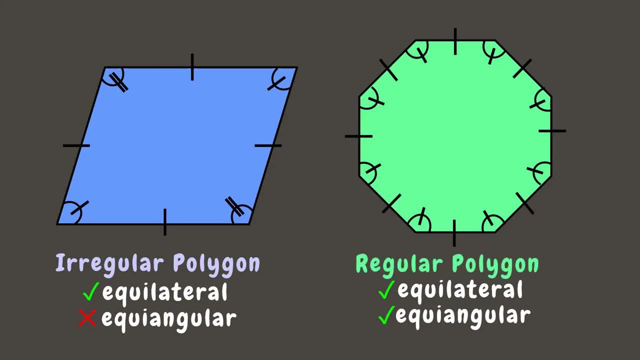 While the other one is the regular polygon, Because it's both equilateral and equiangular. Equilateral and equiangular. The first polygon is a rhombus. We can call this as irregular rhombus, since all rhombus are irregular. 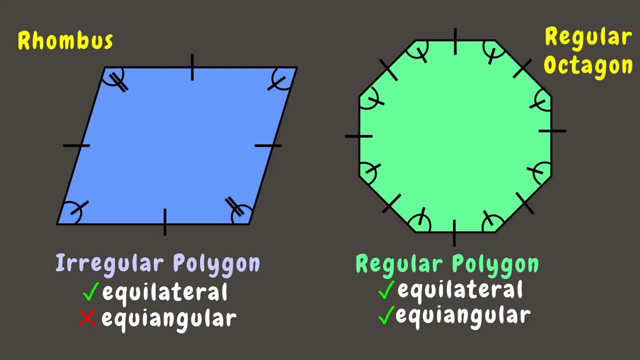 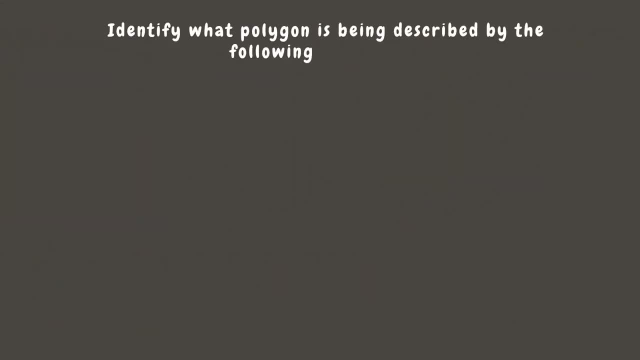 While we can call the other one as the regular octagon, Since not all octagon is a regular polygon. Now let's identify what polygon is being described by the following statements. The first one: a 12-sided polygon where all sides and angles are equal. 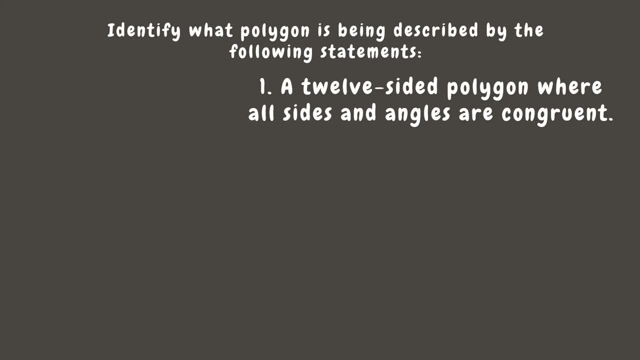 Since all sides and angles are congruent. Since a 12-sided polygon is a dodecagon and its angles and sides are congruent, Therefore it is called a regular dodecagon. Next one: it has four equal sides, where all sides form right angles. 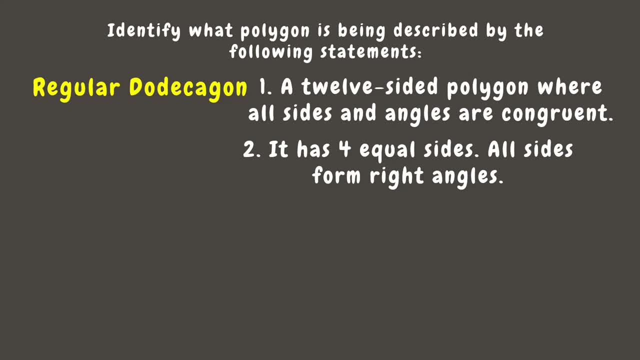 We know that a polygon with four equal sides and four right angles is called square. Remember that there is no such thing as a regular square, since all squares are a regular polygon. Next one, a six-sided polygon with equal sides and equal angles. This one is a regular hexagon. 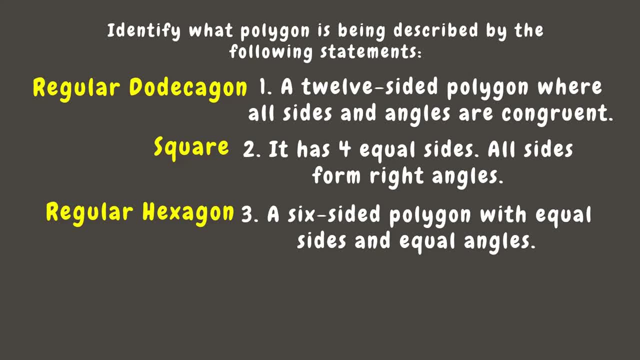 Since a six-sided polygon is called a hexagon and since it is equilateral and equiangular, we can call it as regular hexagon. Last one: a ten-sided polygon where sides and angles are not equal. We know that a ten-sided polygon